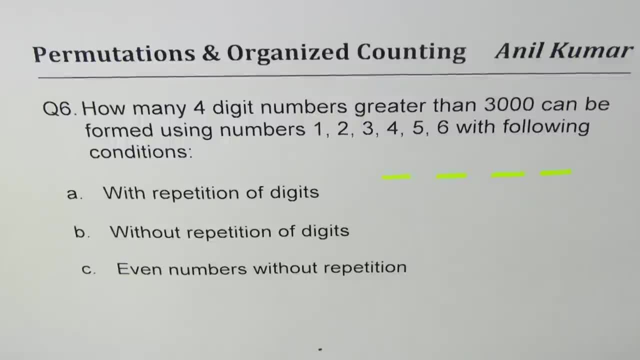 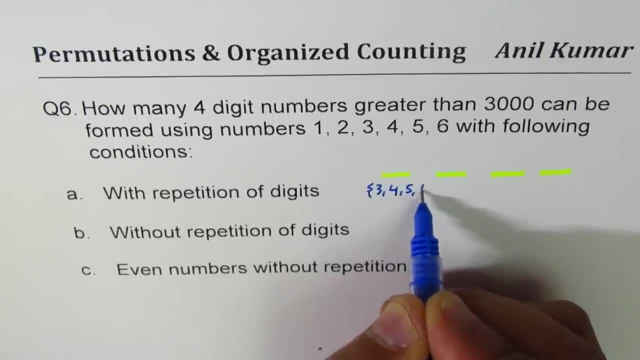 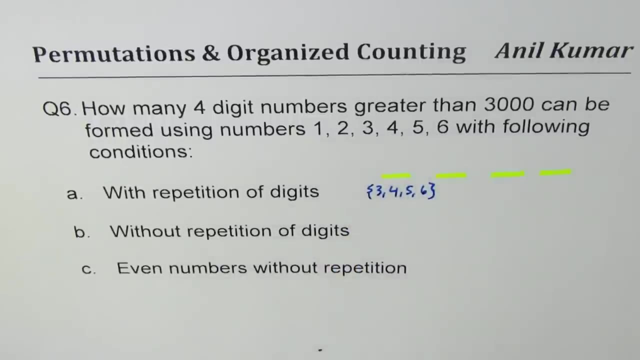 in the first place we could have numbers. let me write down here: 3,, 4,, 5, 6, right? So there are only these four numbers which can take the first place. So let's write down four on the top. So we 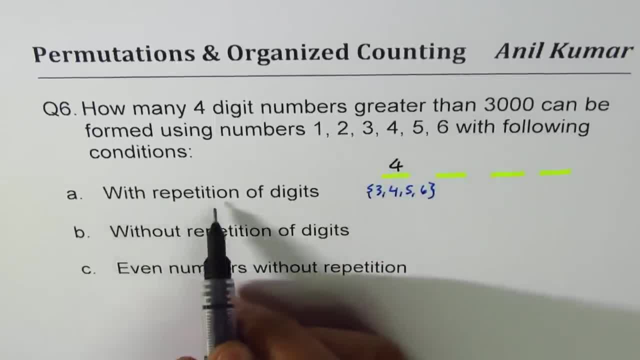 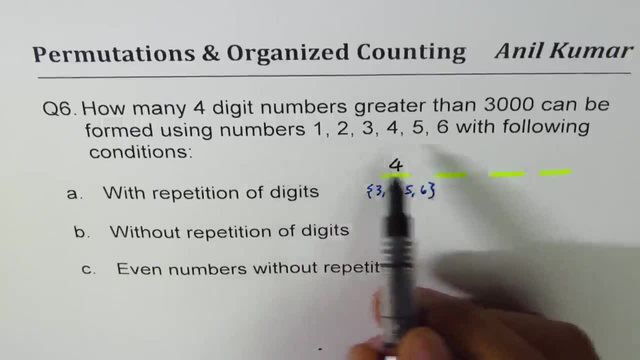 have choice of four numbers, With repetition of digits allowed. that means in the other places we can write down four numbers. So let's write down four numbers. So let's write down four numbers. We can place any of these digits, which are 1,, 2,, 3,, 4, 5, 6 digits right, So 6, 6 and 6.. 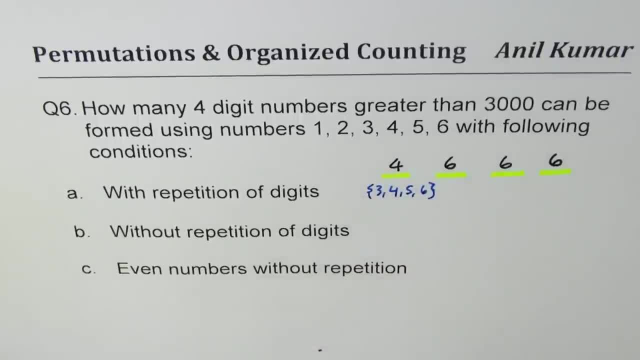 Multiplying them using the fundamental property of counting, we can find how many four-digit numbers greater than 3000 can be formed from these digits with repetition, Is it okay? So let's multiply and get our answer. So you have four times six times six times six, And then you have four times. 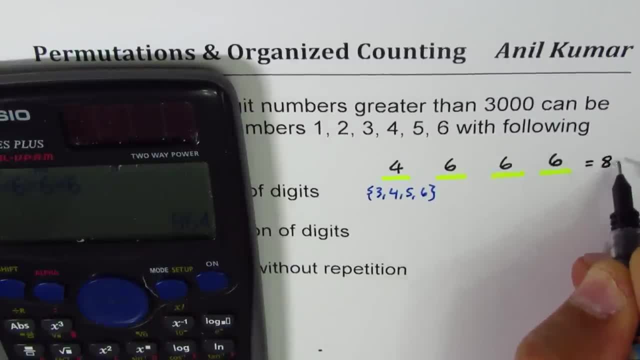 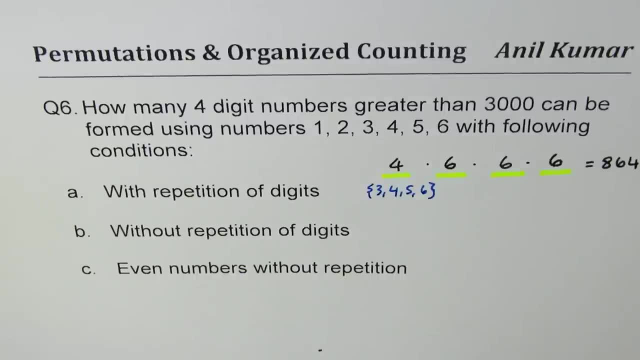 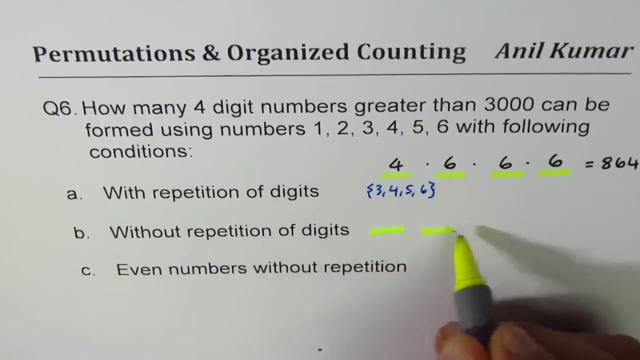 six times six times six, And that is equal to 864.. Is it okay? So we just multiply these numbers to get our answer? Okay, Now let's do the next one, which is without repetition of digits. So it's kind of similar question, but with a major difference. Now we are not allowed to repeat. 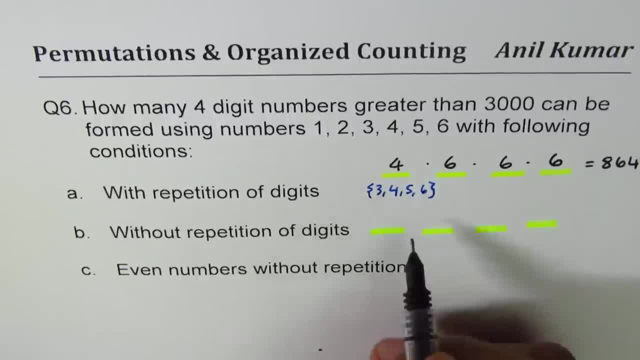 these digits. So in the thousandth place we can only put one of these four numbers. So still, we have only four options. Now, once you put a number here, we cannot place that number anywhere else. So we're left with not six, but five numbers. Do you see that? So we have option. 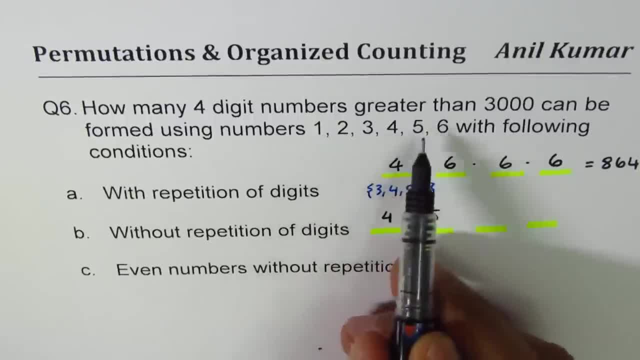 for putting five out of six right. We already put one, So 1,, 2,, 3,, 4, 5.. We've already taken one of them here. Now, once you take two numbers away, then you're left with four choices And 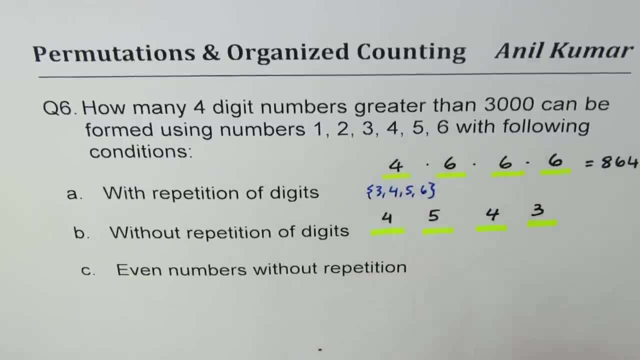 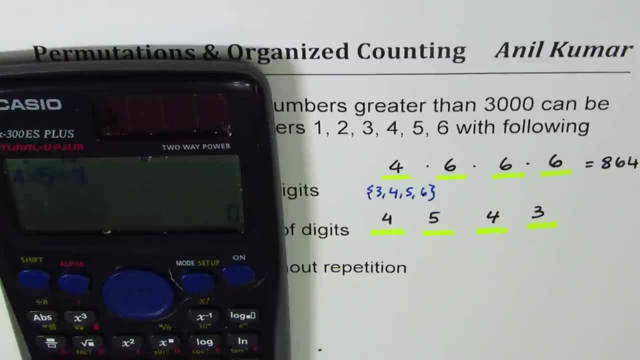 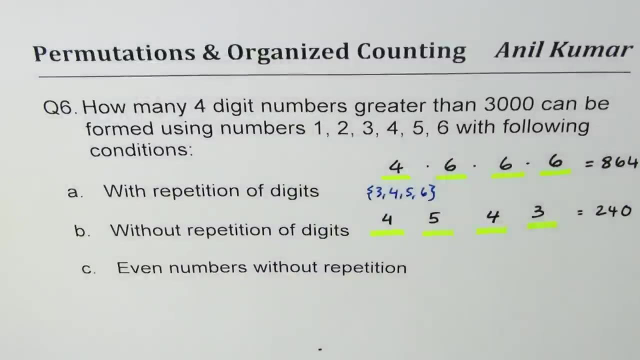 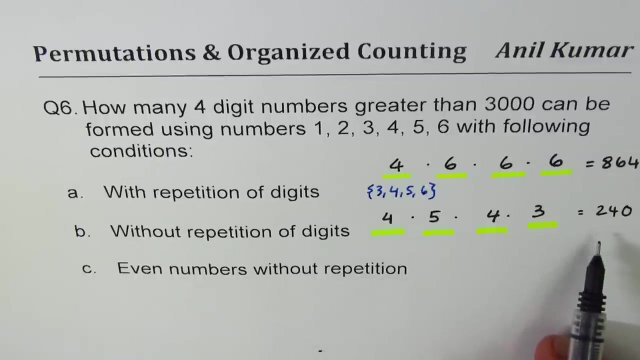 three numbers away from six. you're left with three choices And therefore the number of numbers will be four times five times four times three, And that gives you 240.. So if repetition is not allowed, you cannot use the same number more than once, So you get much lesser options. The 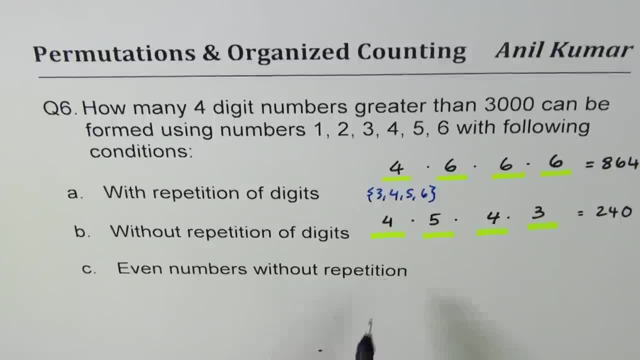 condition is even numbers without repetition, Do you understand? So condition is how many four digit numbers greater than 3000 can be formed using 1, 2,, 3, 4, 5, 6, with following condition, which is even numbers without repetition, right? How do you do this part? Now think about it. If 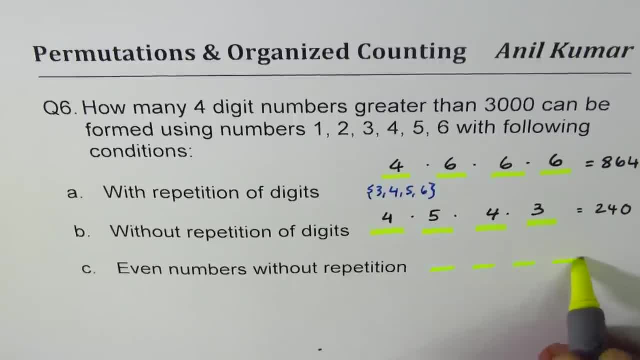 we have even numbers. that means the last could only have even numbers 2,, 4, and 6, right? So we could have numbers 2,, 4, and 6 in the last place. We also have a choice of taking numbers 3,, 4,, 5, 6 in the first place, since the 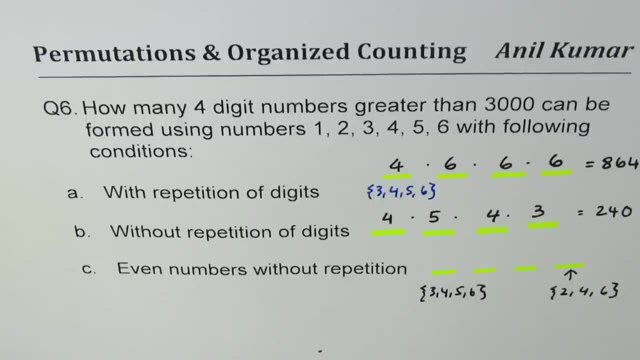 number has to be greater than 3000.. Now, and the numbers cannot be repeated. Now it is not that simple that we just put four here, Because if I put four here, I really don't know which number has been taken. If an even number has been placed, then that even number. 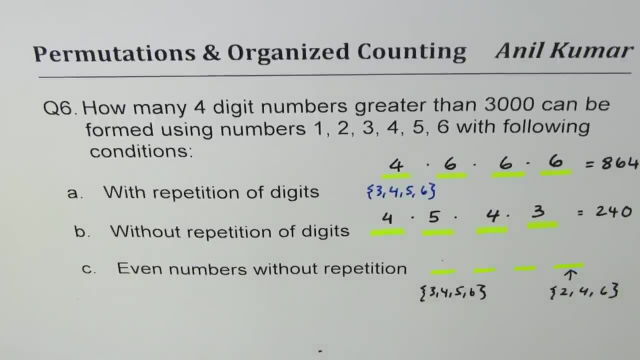 cannot come at the end, Is it okay? So in such cases, what happens? That we should actually look for possibilities based on the last digit. So we have three numbers here possible, So we'll make three different scenarios use, is there okay? so three cases, so that the first case be, let me say, one, two, 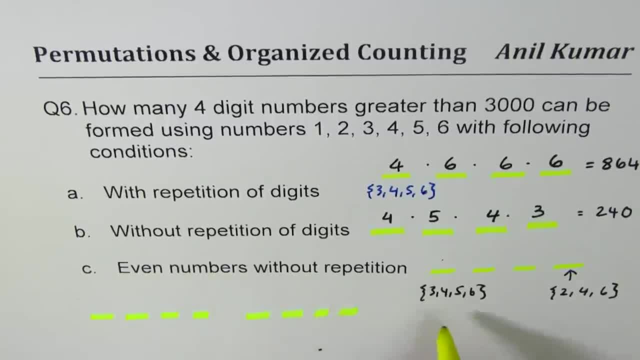 three, four. one, two, three, four, and okay, we'll use this one as our third case, is it okay? okay, so we can place two in the last digit. we could place four in the last digit, or we could place six in the last, is there? okay, so that is our third. 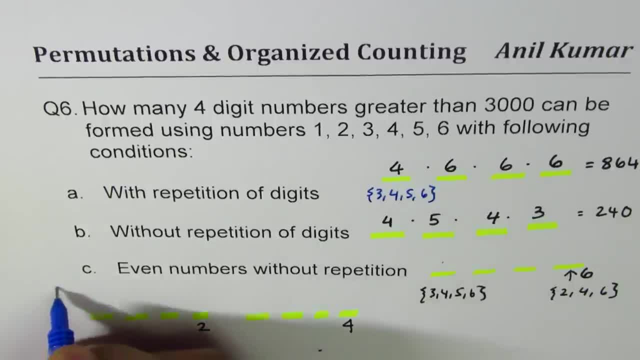 case. so what we are saying here is that this is case number one, case number two and case number three. now, these are all our conditions if you place two right or four or six right. so they will add up all these options. add up. now let's look. 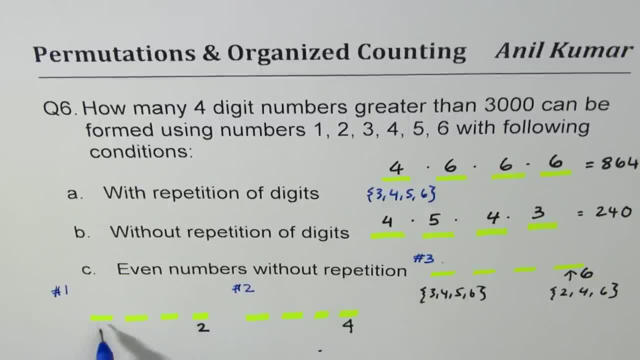 into the first case. if I place two here, my choices for the first place are not limited, because three, four, five, six does not include two, is it okay? so I have four choices, so let me put four now. I already consumed two numbers out of six, so we are one, two, three, four, five, six. 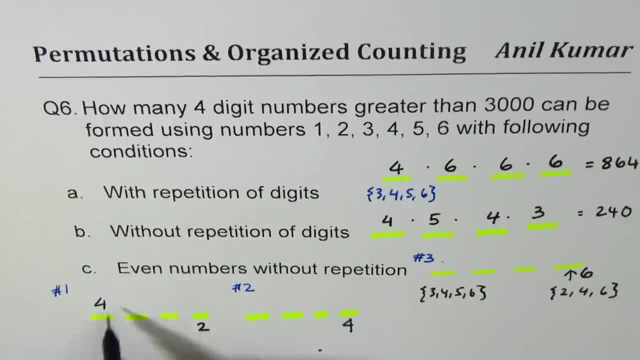 since I have taken away two numbers, I am left with four, and once I take the third one, I am left with three numbers, right. so we have a choice of four times four times three. if you multiply these, you get three, three, twelve times three, forty eight, right. so this gives you forty eight. 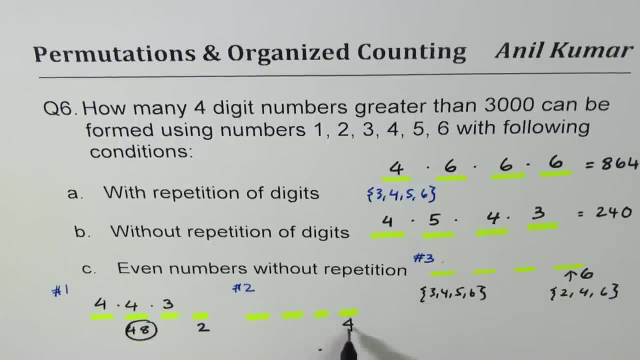 in the second case, if I place four, then my choices for the thousand place are limited. we have only three choices left right. once we have placed these two numbers, six take away two is four, so the center positions. we have options of four and three, as before now, 9 times 16, so let's multiply so 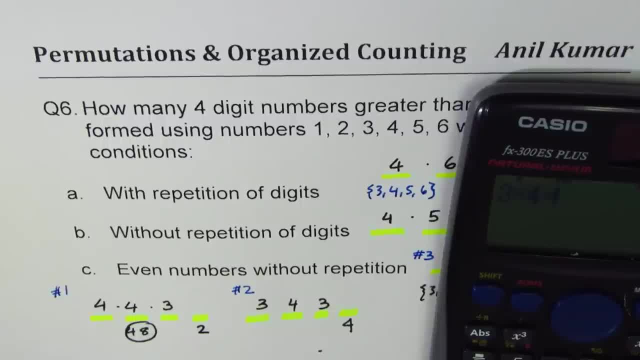 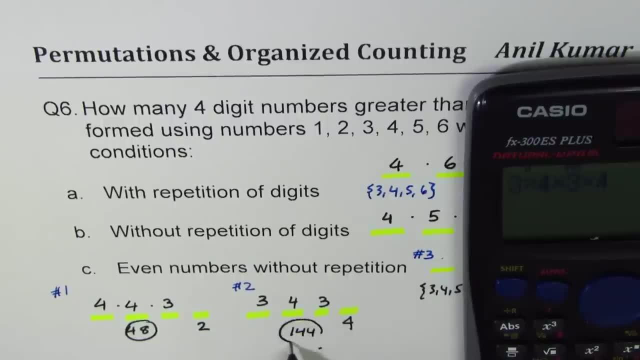 we have three times 4 times 3 times 4 as our answer, which is 144. so here get we get 144, I'm sorry. three times 4 times 3, sorry, let's redo it. three times 4 times 3 here 36, sorry. 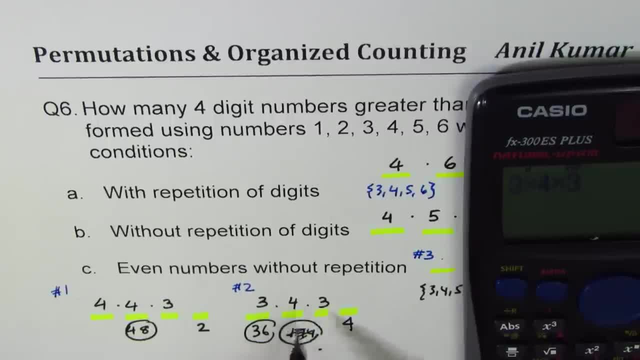 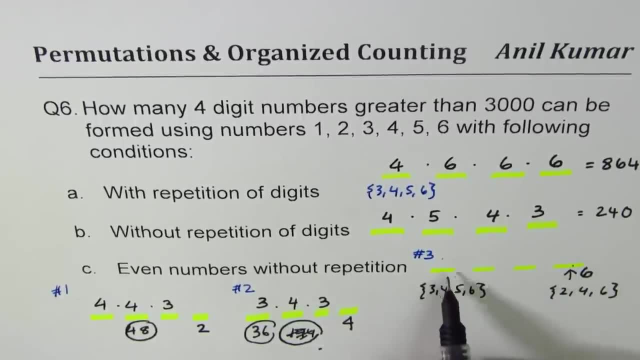 so the choices are 36. 3 times 4 times 3, is it okay? Now, in the last case, if I place 6 here, I cannot place 6 in the first position. so I have choice of 3 numbers. 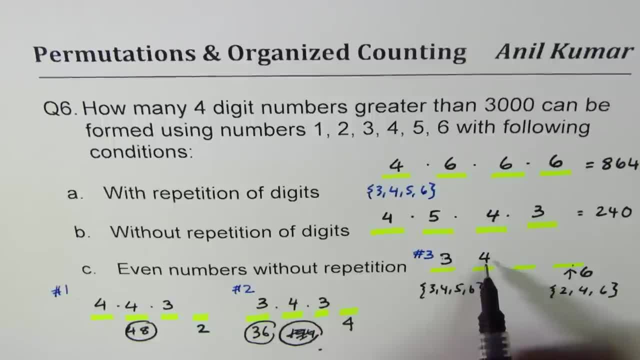 I have placed 2 out of 6, so I am left with 4.. Once you place the third one, you are left with 3.. So we have 3 times 4 times 3, which is again 36.. So for even numbers without repetition greater than 3000, our answer should be 48.. 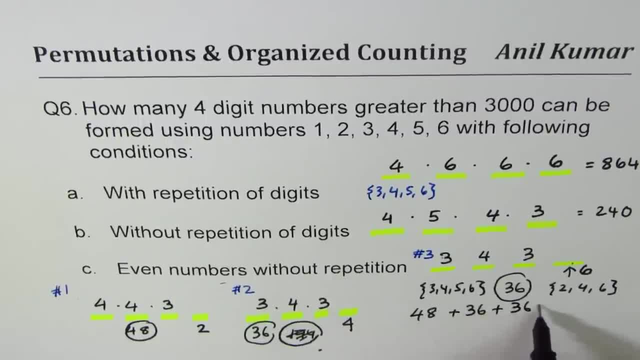 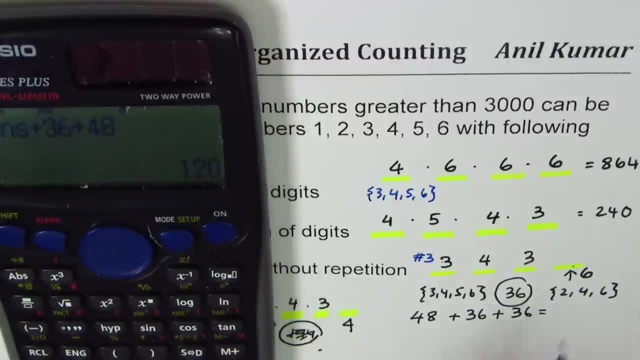 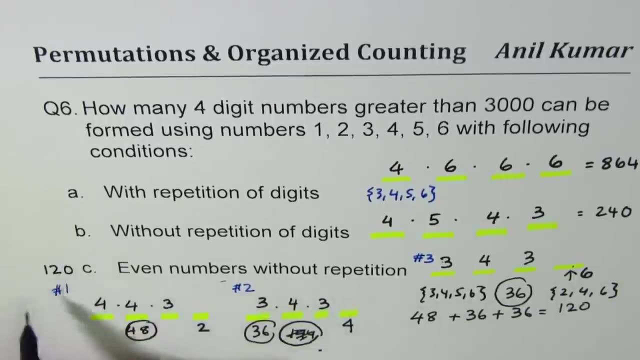 Plus 36, plus 36,, which is, let's add this, 36 plus 36 plus 48,, which is equal to 120.. So there are 120 combinations for part C. So 120 is for part C, 240 for part B and 864 for part A.